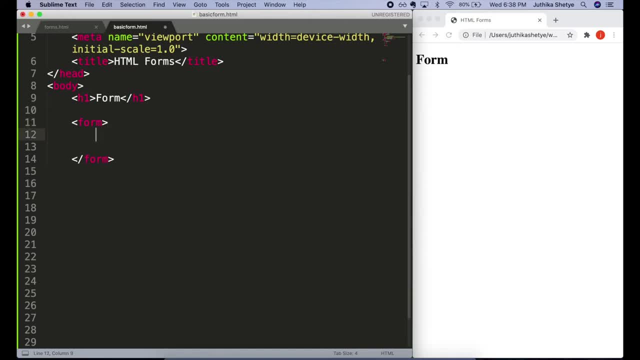 And that's because the form element is a container element, just like a table section or a footer element. It is a holding place for a file And it is also a holding place for all other form elements. Now let's make the two fields in our signup form: name and email. 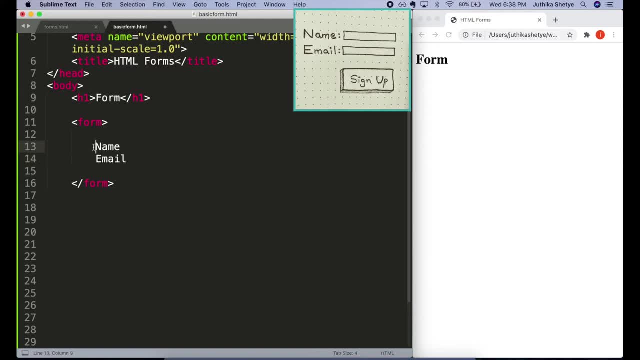 We don't keep these hanging just like that in the form. We have to put them inside some element. So we'll make these form elements into labels by using the label element. Then we want to add the actual places or boxes where someone will type their name and email. 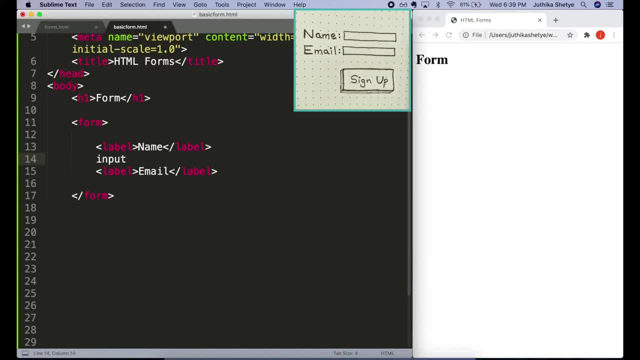 So we'll add the actual places or boxes where someone will type their name and email, and we do that with the input element. it specifies an input field where the user can enter data. it is an empty element, meaning it does not have any content or closing tag, but it is the most. 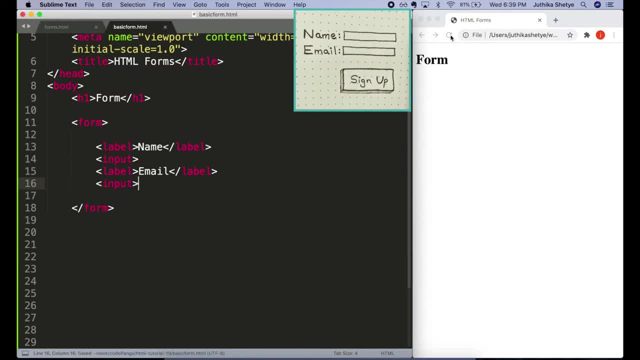 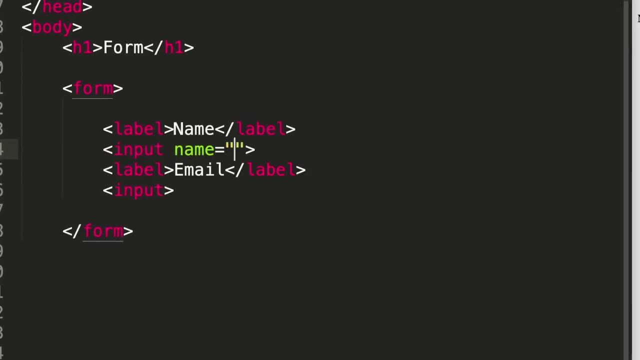 important element in a form. this is where all the magic happens. the browser puts a whole lot of complex functionality in this tiny little box. now, although it looks fine, the input field is not yet complete. each input field must have a name attribute for the form to be submitted to the. 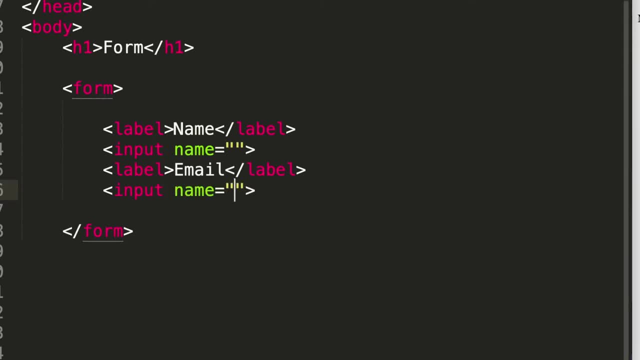 server. if the name attribute is omitted, the value that is written in the input field will not be sent at all. well, we are not going to actually send anything in this tutorial. it is all back-end stuff which you will learn later if you decide to study back-end development. but for now let's just 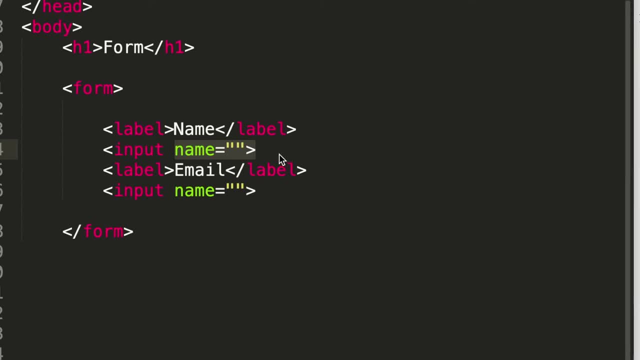 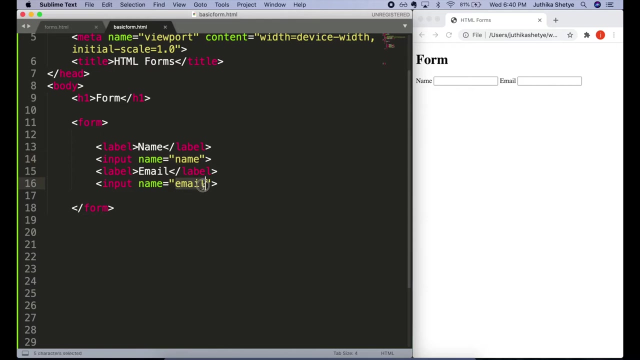 understand that this name attribute is very important for all the forms elements. so let's add name equals name to the first input element and name equals email to the second. we can call this whatever name we want. name equals first name or whatever we want. next, we also need a button on our form that people can click to submit the form. for that we are going to. 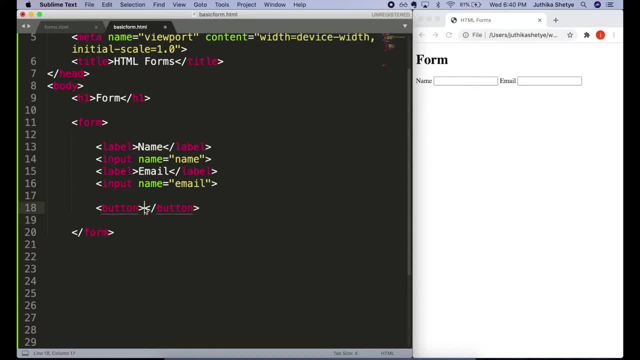 use the button element. it has both an opening and closing tag, and whatever words we put as content in between the tags are the words that will display on the button itself. let's write sign up here. if you look in the browser, we now have a simple sign up button in our form also right now. 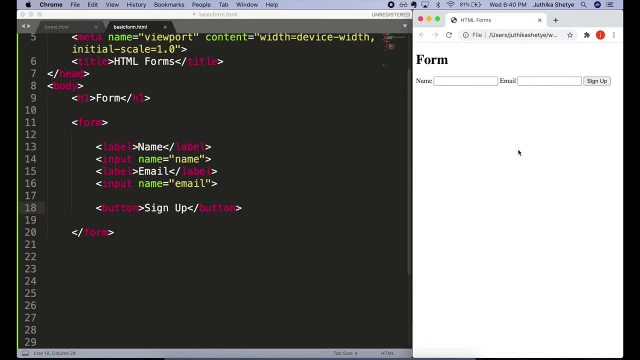 the form looks kind of ugly, but the styling can be easily changed later using css. in this tutorial we are going to focus only on html. now let's see what this button does. let's type something in these fields and then click the button. well, right now the button doesn't do anything. it doesn't submit. 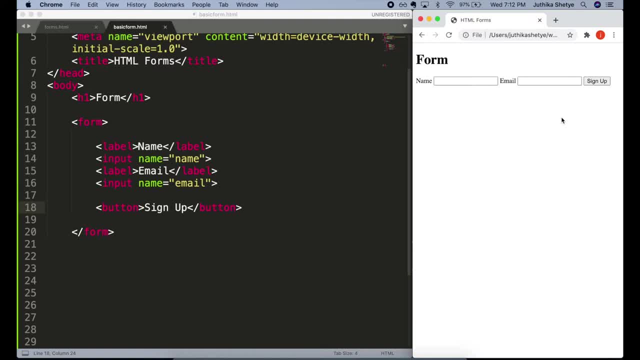 our form anywhere because we haven't added any back-end code. but again, we are just going to focus on the html part in this tutorial. now, if you see the code, the label element and the input element are just sitting next to each other. they aren't actually connected to each other. people who do not 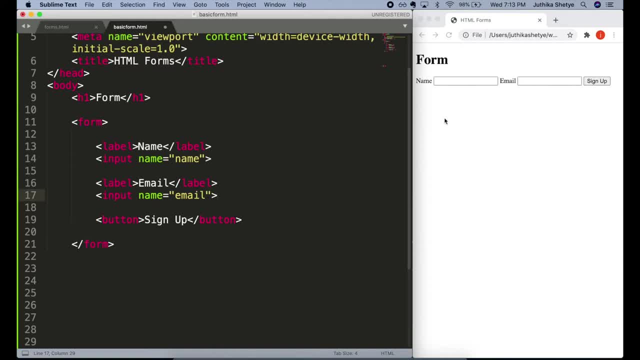 know how to connect them professionally, like we do with a screen that they can see or a mouse to click on an input field, will not know that this label goes with this input. so in order to connect them, we have two options. first, we can add a for attribute to the label and an id attribute to the 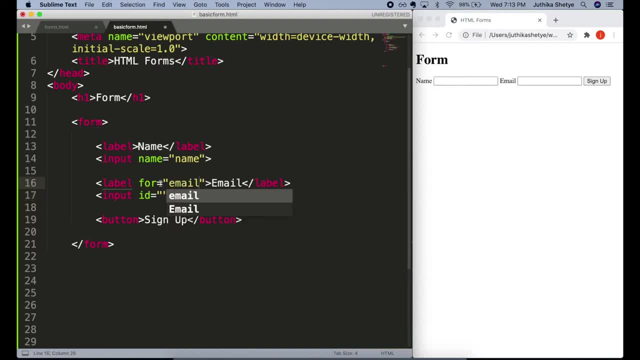 input with a matching name, let's say for equals email on the label and id equals email on the screen, as long as the two names are the same. or the second option: we could wrap the label around the entire input element, which clearly communicates to the browser that this label is for this input. 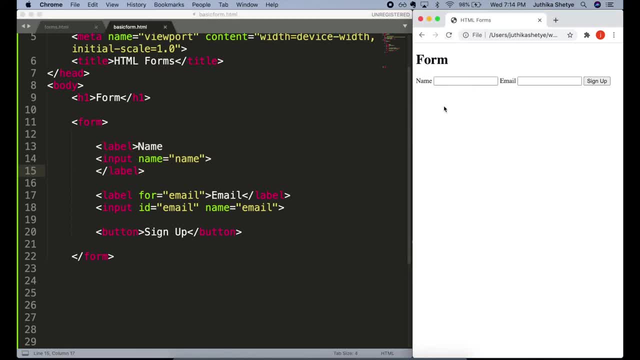 field. both options work the same. to test if they are actually connected, we can go back to our web page and click on the label. see how, when i click on the label, my cursor automatically shows up in the box and there is a focus state or a blue ring around it. that's what we want. next, i want to bring 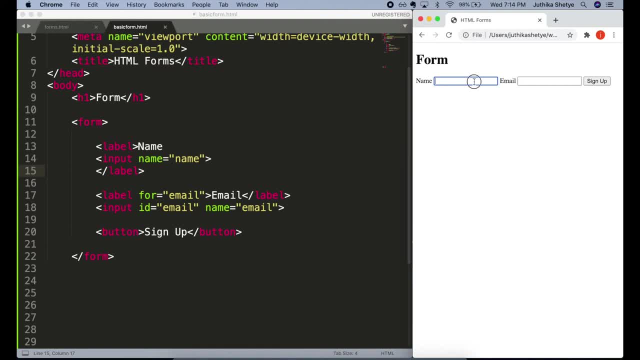 your attention to another problem in our form. when i type inside these two input fields, i can type anything i want and the form will accept it. but we want people to type an email in this field and not just any text. so how can we fix that? well, for that we use the type attribute in each of these fields. 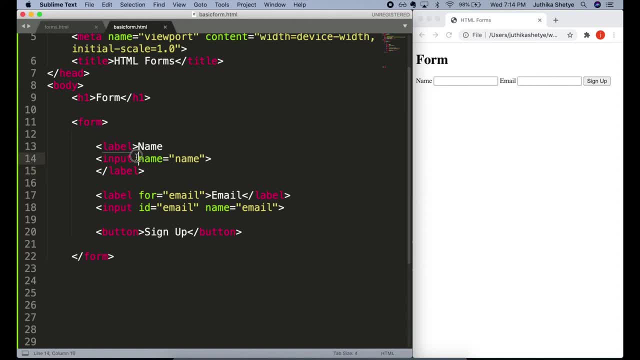 for the input elements. for the name field, we will collect text which is the default type of the input element. if you don't write any type attribute here for the name input element, the browser will assume that it's the type equals text. so we don't have to include it. but as a good practice and for 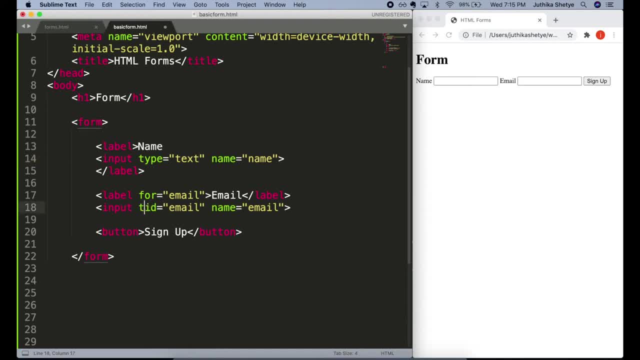 completion's sake, let's write: type equals text. then for the email input, type equals email. now let's go ahead and test this. so a name here and some text here and hit sign up, so you can see a warning immediately popped up here asking us to type an email address- that's awesome- by writing. 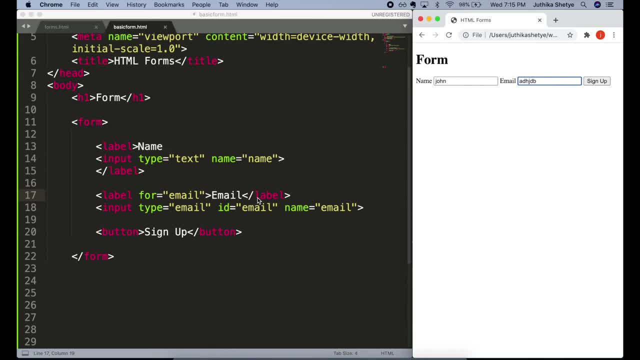 just the correct type attribute inside the input element. we are getting validation for free from the browser now we also want the browser to know that this button on the page is a button to submit. we might have multiple buttons on this form later and we want to let the browser know. 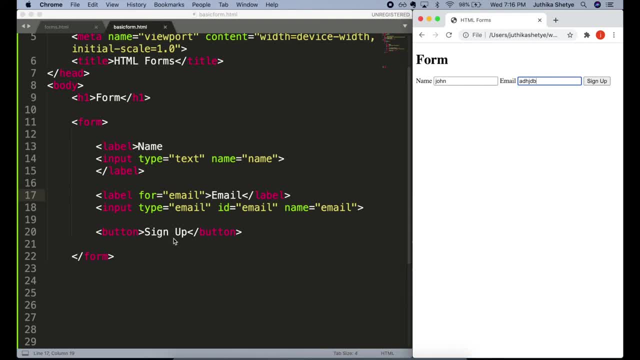 which button to activate when a user hits the return key or the enter key on their keyboard, because sometimes people use the return key to submit instead of using a mouse to click the submit button. so we will just write: type equals submit for this button element. there's another way that you can make a submit button instead of using the button element. 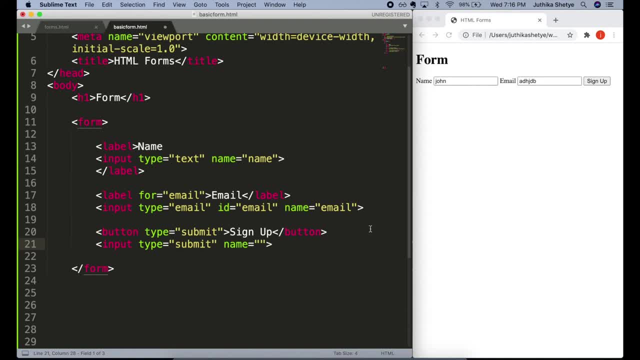 you can use the input element and the type attribute here will be submit, name, as usual, anything you want. let's just write submit and then the actual text that will be seen on the button will be written inside a value attribute. so let's write submit here and you can see in the browser. we have this other button and it works exactly like the earlier one. 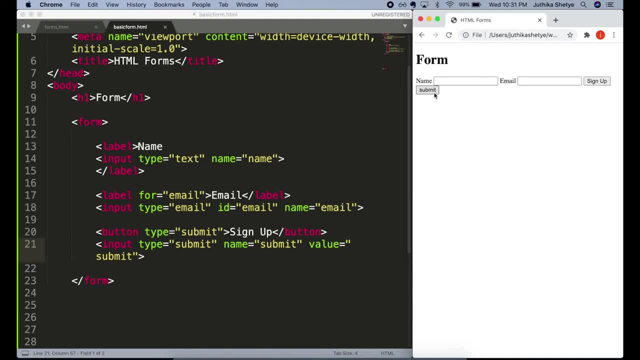 next, we can further enhance our form by making any of the input fields compulsory before submitting the form. right now, the browser seems to be accepting the form, even if we type only one of the fields. so, to make a particular field compulsory, we can add the required attribute. 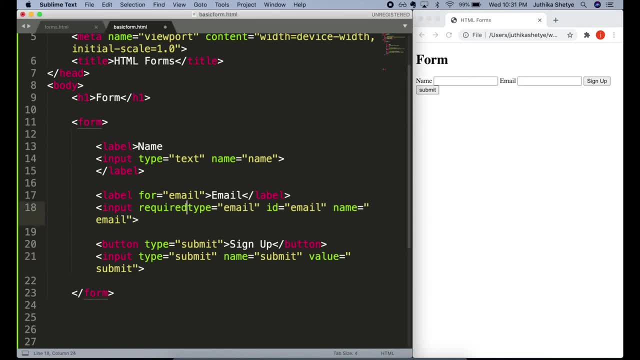 in its input element just the word required. now, if i try to submit the form without filling out the email, you can see the browser is insisting that i fill out the email field by showing me a warning pop-up. it won't let me submit the form without filling the required field. 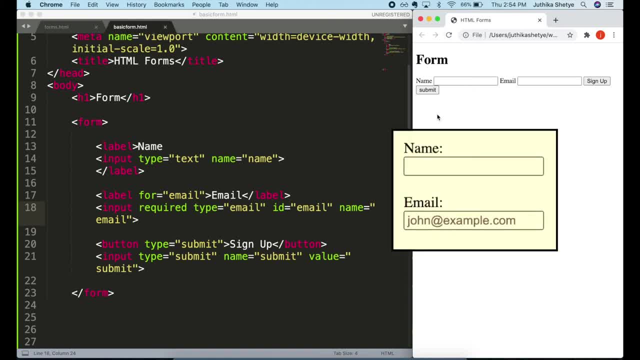 lastly, let's look at including some placeholder or a default value in our input boxes. it is like a suggestion to our form users of what should go into that particular input field. to do that we use the placeholder attribute and inside the codes we type in the suggestion that we want the users to see in the input box. 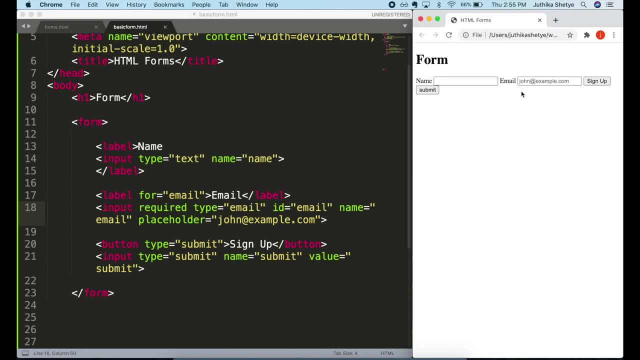 you can see that now the suggested text appears in the box. it's light gray by default, and as soon as i start typing into this field, the placeholder disappears. that's important. users should not have to keep erasing the placeholder text in order to write their own email addresses or other data. 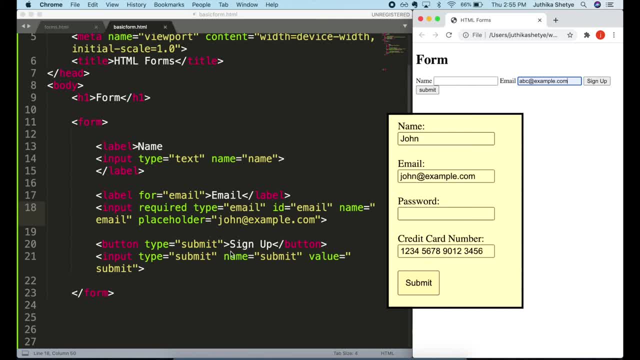 if you in fact wanted to pre-populate the input field with real content instead of just a suggestion, like you see with many forms nowadays that auto complete with the user's name, address, credit card numbers, then you must use a value attribute instead of the placeholder attribute. 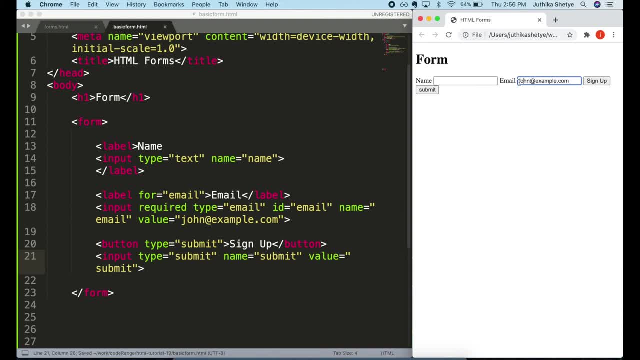 so now, if i click in this input field to type my own email address, the pre-populated one is in the way. i have to manually erase it, which will be happening shortly for the falls. when that Authority poll is completed. manually erase it to put in my own. It doesn't disappear, like the placeholder, And that's. 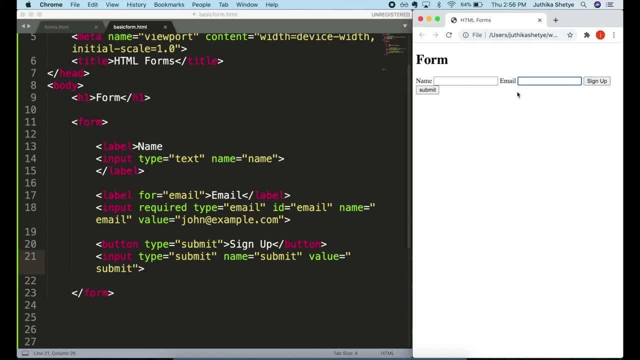 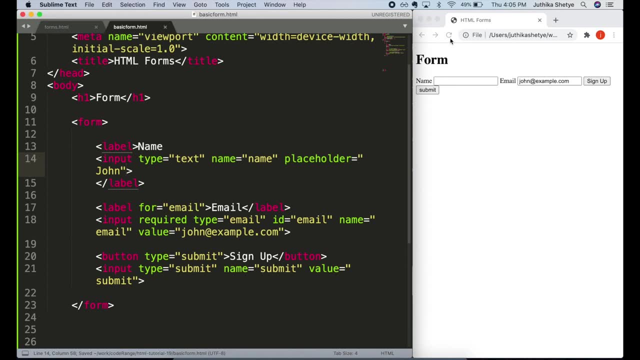 because the placeholder is just a suggestion, whereas the value is real data. So if I were to submit this form with a placeholder and the value attribute on two different inputs, then the input which has the value will be the only data that will get submitted with. 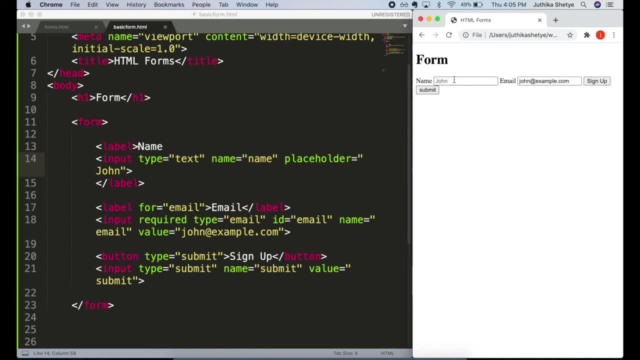 the form. after clicking the submit button, The placeholder does not go through. It's basically nothing in that input And that's it. These are the few of the many parts of a form. Right now, what we have is just a basic form, But there's much more to forms.